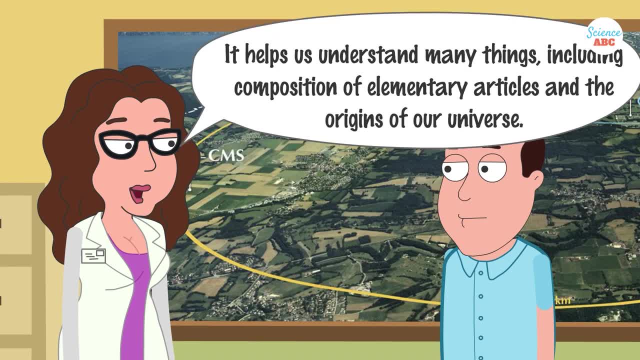 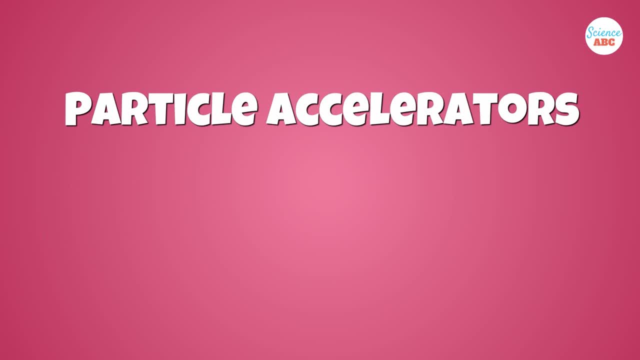 only help us understand the composition of the elementary particles in question, but also supplement our knowledge of our universe's origin immediately following the big bang. Particle accelerators can be broadly classified into two categories: linear accelerators, also called line-axe accelerators, and circular accelerators. Line-axe accelerators, also known as linear, 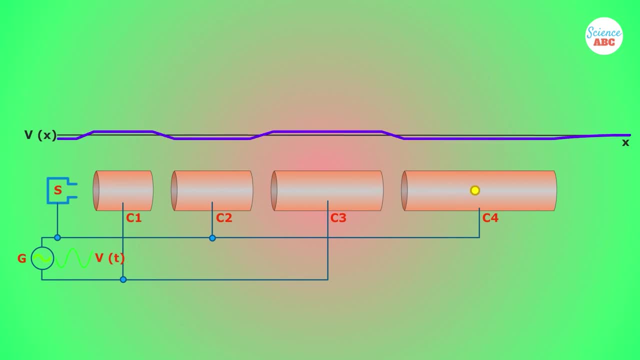 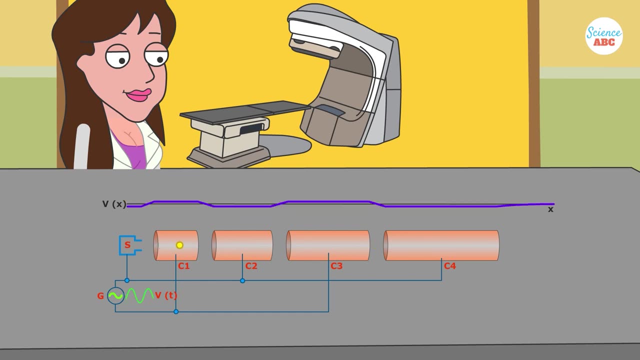 accelerators can be classified into two categories: linear accelerators and circular accelerators. A linear accelerator accelerates ions or subatomic particles to a very high speed using a strong electric field along a linear path, hence the name: linear accelerators. A circular accelerator. 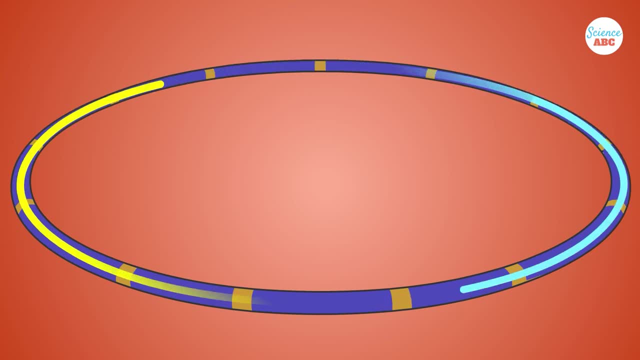 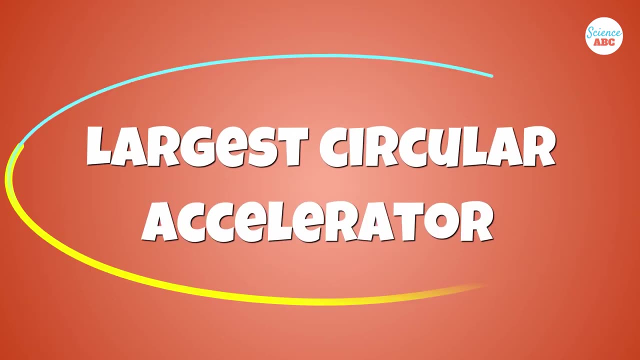 in contrast, accelerates elementary particles along a circular path to finally smash into a target or other incoming particles from the opposite direction. The largest circular accelerator in the world is called the Large Hadron Collider, or LHC, which is located at CERN near. 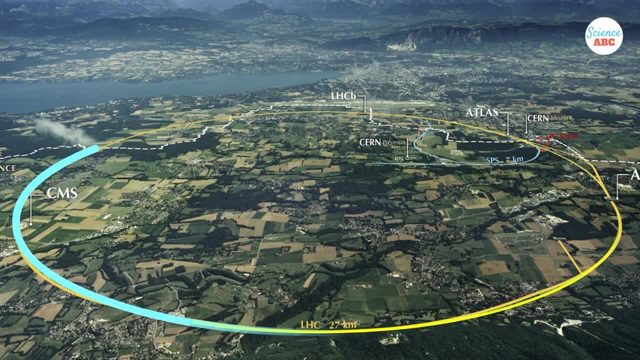 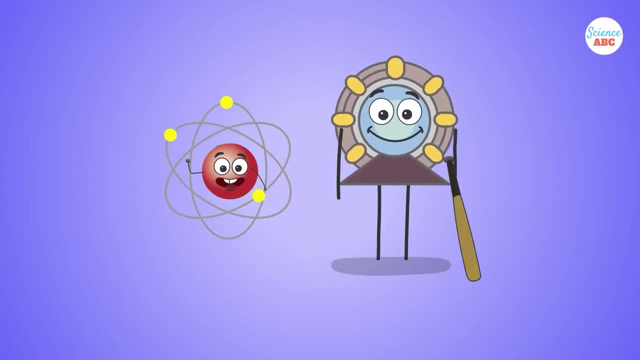 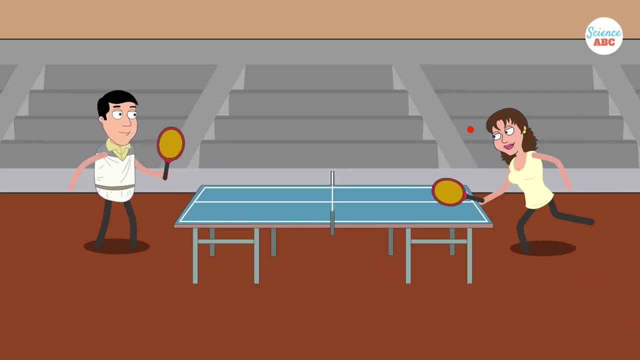 the French-Swiss border. The circumference of the accelerator is nearly 17 miles, or 27 kilometers greater than the length of Manhattan. Circular particle accelerators are sometimes also referred to as atom smashers, as they smash subatomic particles into each other. The basic working. 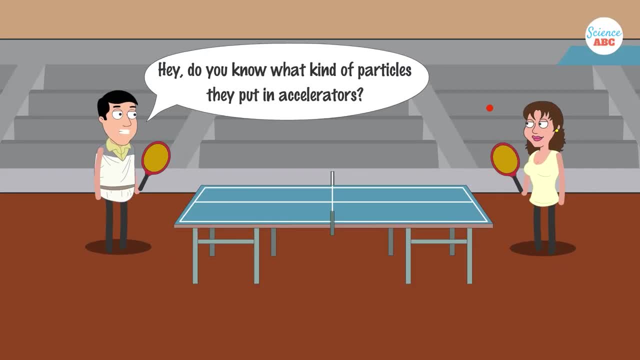 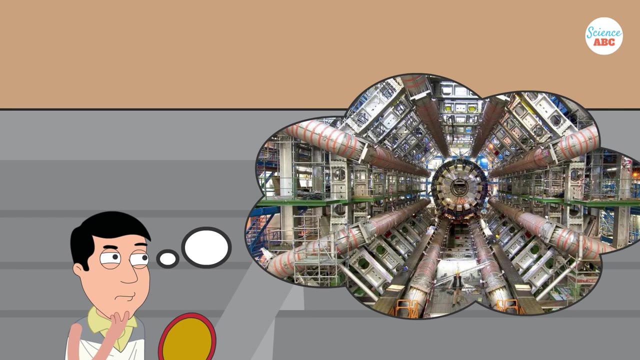 principle of all particle accelerators remains the same: They contain a particle source that provides elementary particles. Although a particle accelerator commonly accelerates protons or electrons, it can accelerate other particles. The LHC, for example, can accelerate the nuclei of argon, xenon or lead. 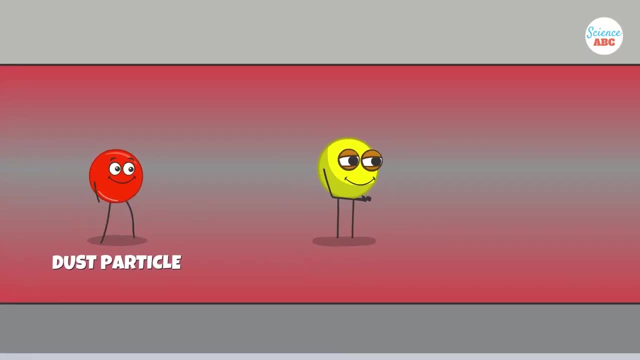 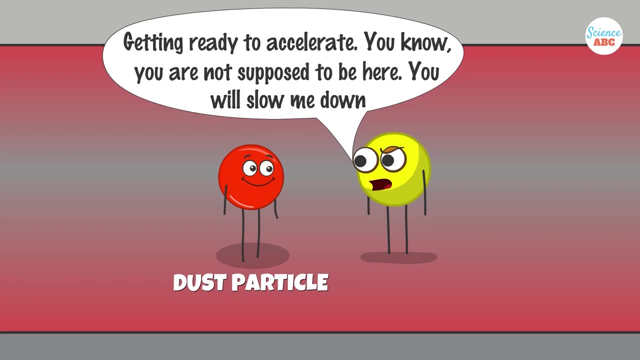 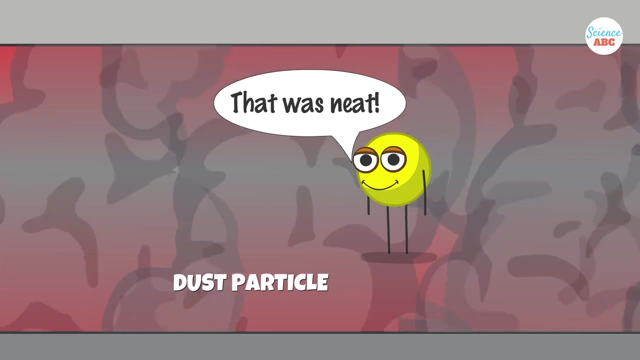 atoms. This beam of elementary particles travels inside a metal beam pipe which maintains a vacuum inside. It is critical to ensure that the whole beam setup is devoid of air and dust particles, so that accelerated particles can travel unimpeded and achieve speeds close to the speed of light. 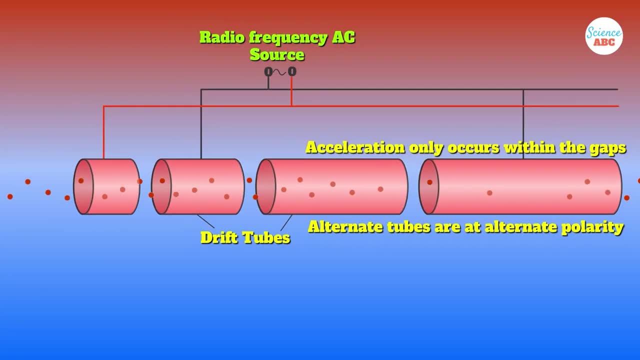 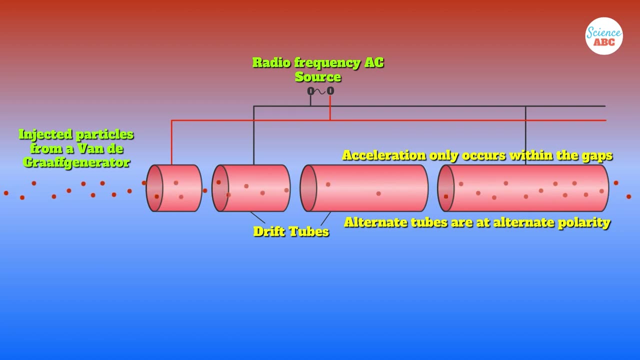 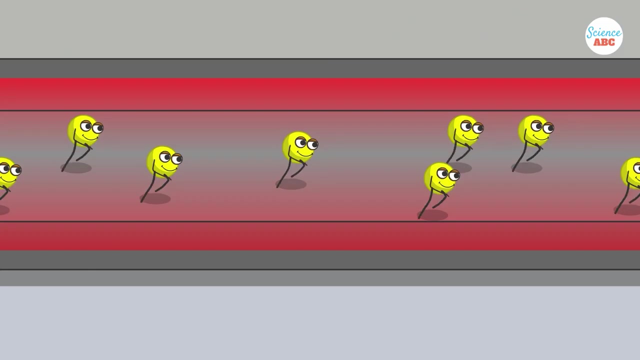 There is special equipment placed around the accelerator that produces strong electric fields. These electric fields allow the particle to achieve such high speeds. They switch from positive to negative at a given frequency, creating radio waves that push and accelerate particles. There are also numerous electromagnets placed along the length of the accelerator. 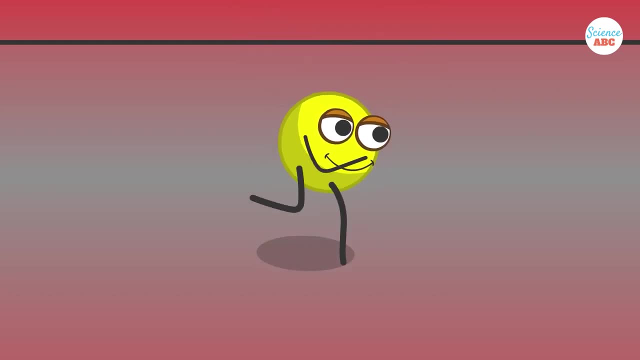 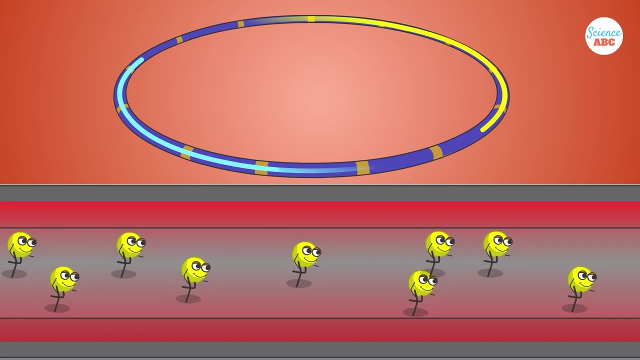 Their primary job is to focus the beam of particles as they accelerate and keep them locked in a circular path within the metal beam. As the particle races extremely fast around the accelerator, it gains more and more energy with each turn. In the LHC, for example.